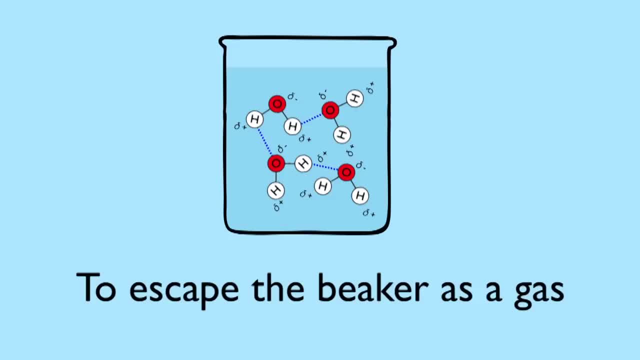 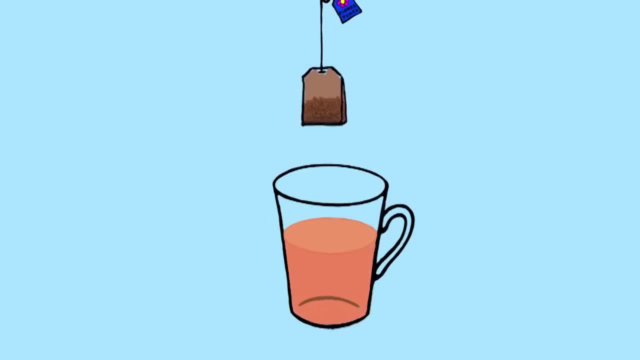 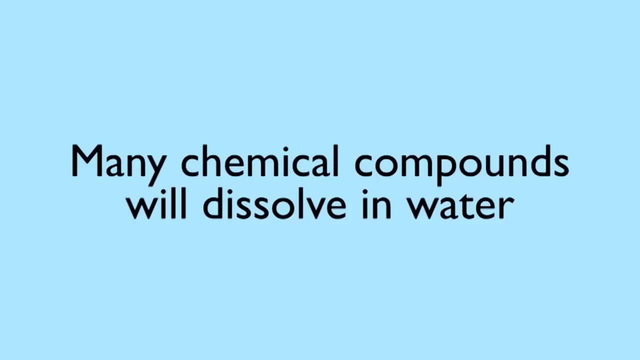 the hydrogen bonds and escape from the beaker as a gas. Water is a very good polar solvent, so good it's often called the universal solvent. That's a bit of an exaggeration, but it's certainly true that many common chemical compounds will dissolve in water. Here's just a few: Hydrochloric acid. 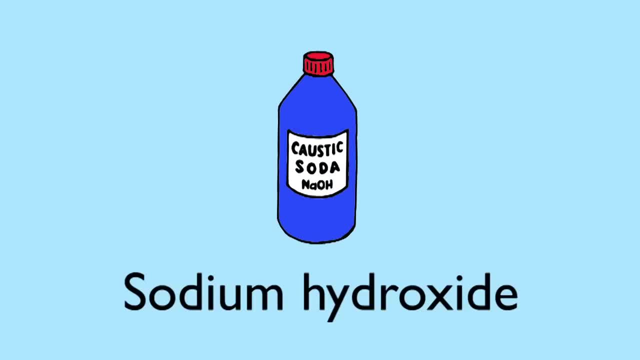 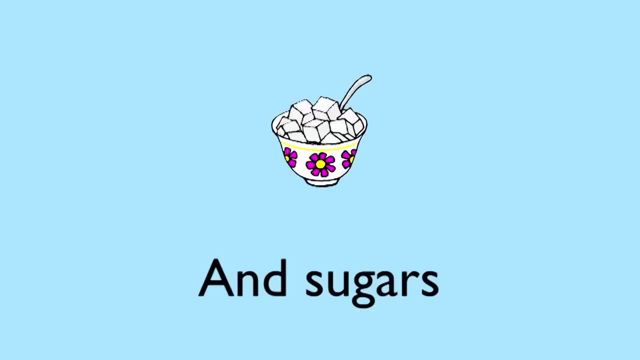 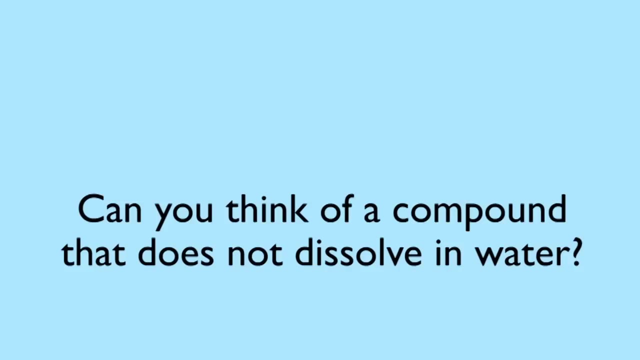 and many other acids, Sodium hydroxide, along with other bases, Soluble salts such as table salt, sodium chloride and sugars. Here's a challenge, though: Can you think of a large and important type of compound that won't dissolve in water and instead floats on its surface? More importantly, 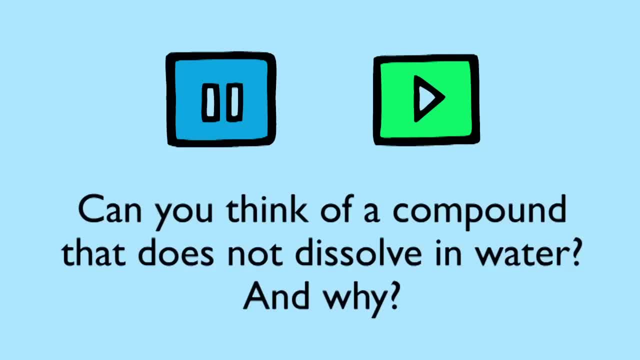 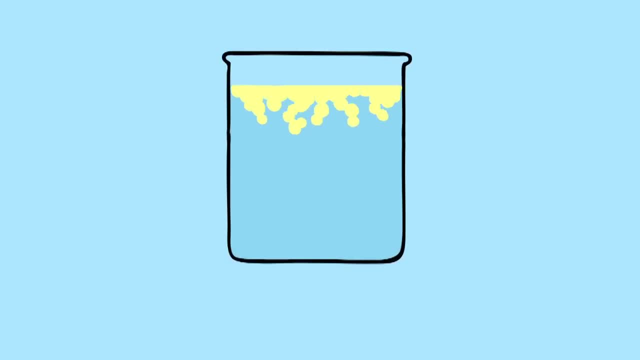 pause the video, think carefully and resume when you've got the answer. Well, the answer is lipids, or, in plain English, oils or fats. They don't dissolve in water because they're non-polar and therefore hydrophobic, meaning they don't like mixing with water. 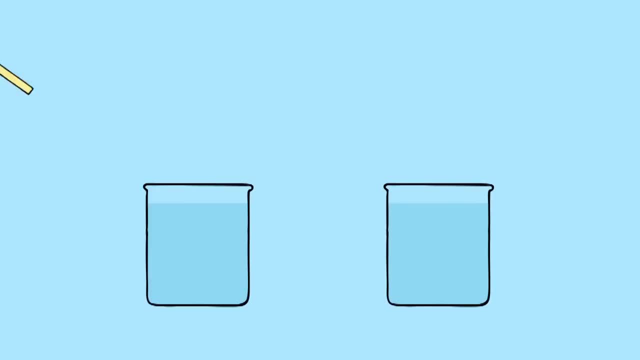 One of the most unusual qualities of water is that it can act as either an acid or a base. A water molecule can either accept a proton and become a hydronium iron with a plus one charge, or donate a proton and become a hydroxide iron with a minus one. 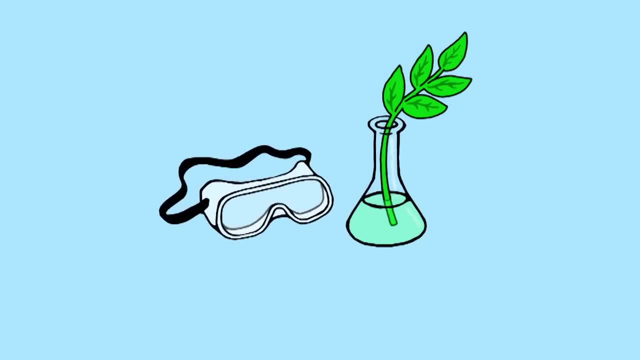 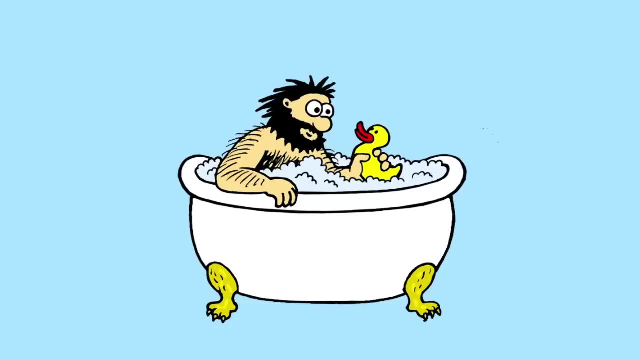 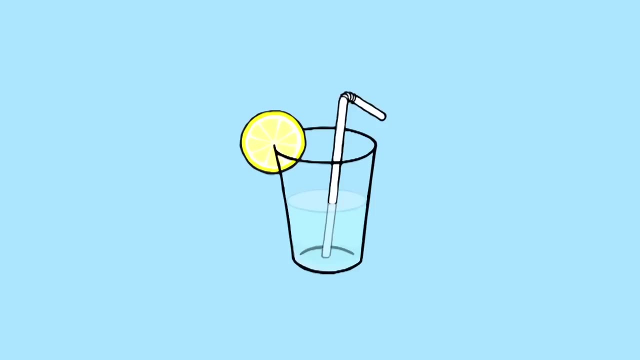 charge. This is one of the reasons why water is so useful in all sorts of organic chemistry reactions. We already use water for bathing, laundry, many industrial processes and, of course, drinking, But perhaps even bigger things lie ahead. You see, many scientists all over the world are working on. 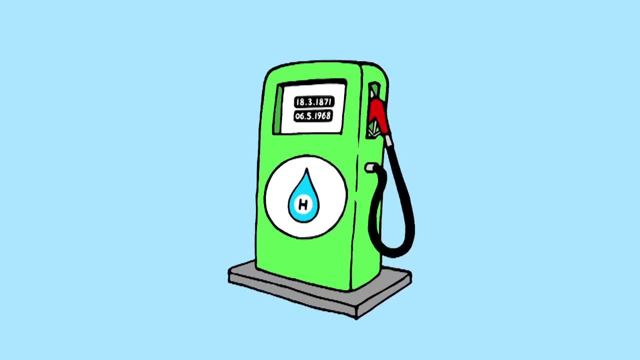 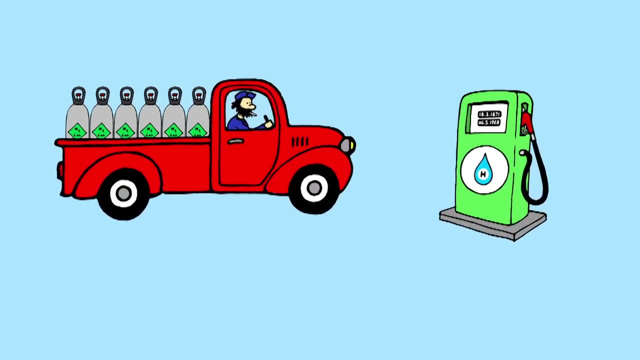 using hydrogen as an alternative fuel source. We know it works for this purpose, but there are problems with storage, transportation and refuelling that are holding us back. Nonetheless, a lot of people believe that in the not too distant future, many of our machines and industries will 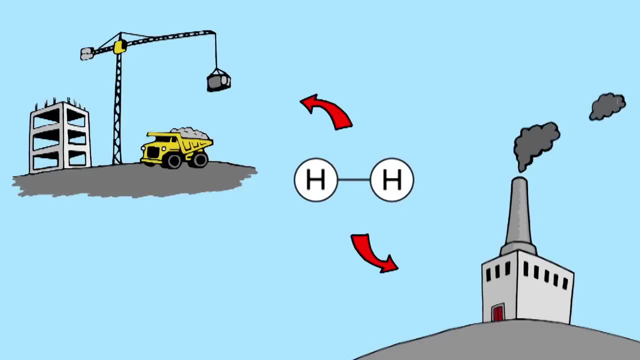 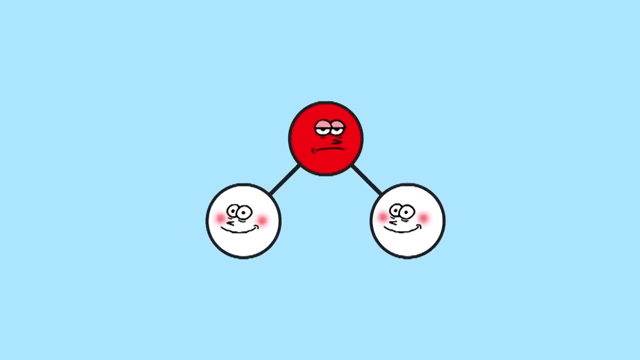 be powered not by hydrocarbons but hydrogen gas. And where are we going to find an almost limitless potential source of hydrogen to use for these purposes? You guessed it: water molecules.